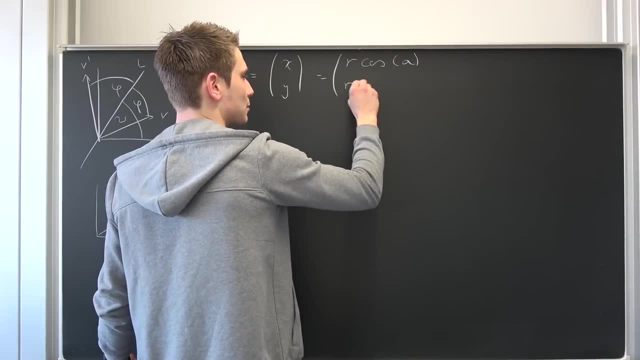 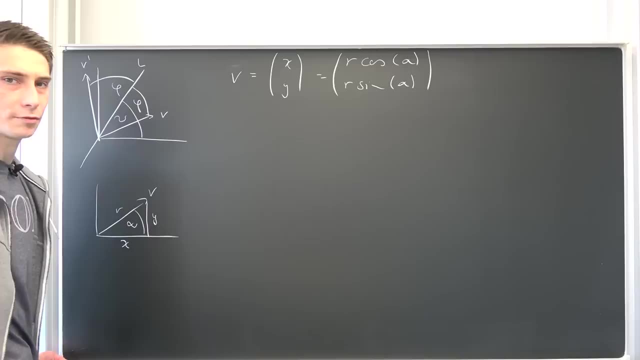 times the cosine of alpha, and down here we have r times the sine of alpha. Now we want to take a look at our vector v. This is our new vector v prime that we are going to get. So, for example, our new vector v prime. 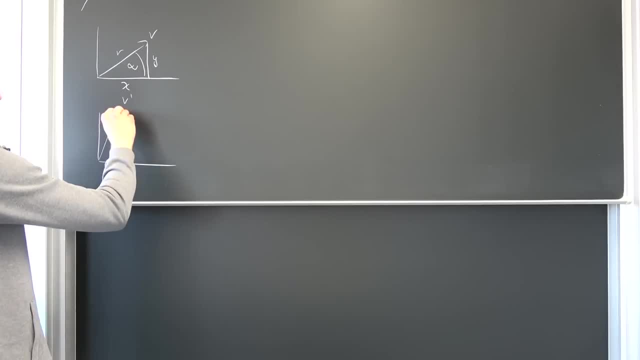 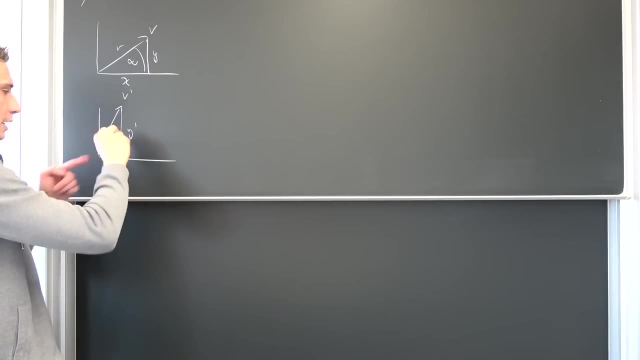 is going to be up here, it really doesn't quite matter- and it's going to consist of some y prime coordinate and some x prime coordinate. also, we have a big angle in between here. let's call it gamma, for example. okay, so that's our angle, gamma being enclosed by the x-axis and the v prime vector. 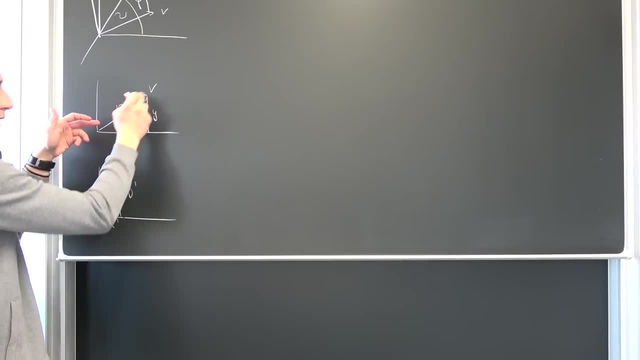 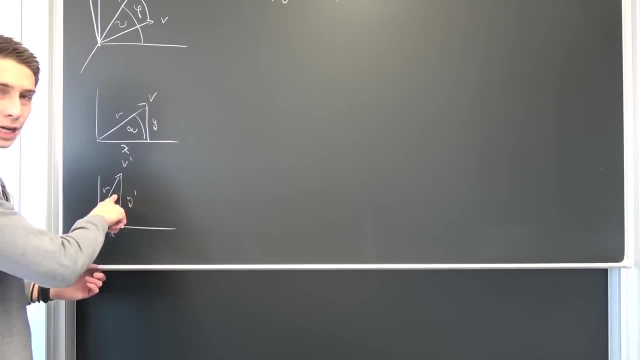 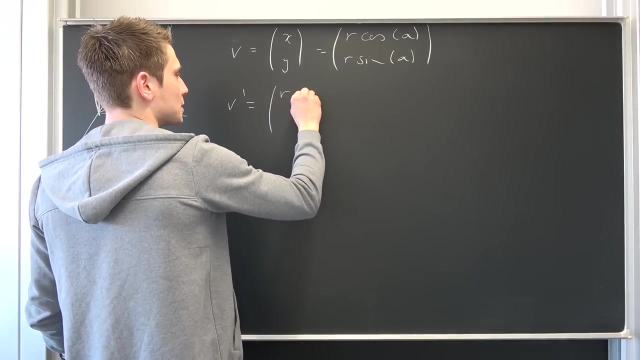 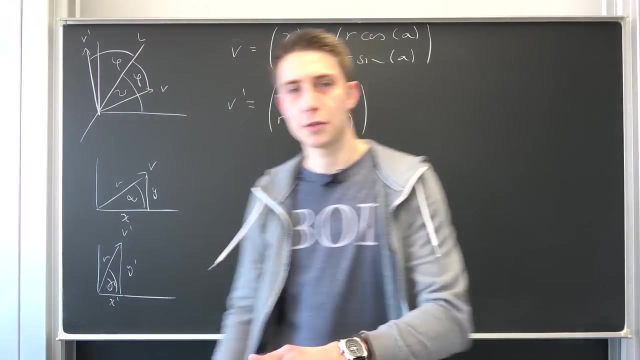 if we just reflect this vector, our magnitude really doesn't change. it's just the same magnitude, just with our um, just like with our reflection matrix. meaning once again we have for v prime, then it consists of some x prime and y prime coordinate, namely this: r times the cosine of gamma and r times the sine of gamma. Now we have to do some playing around. 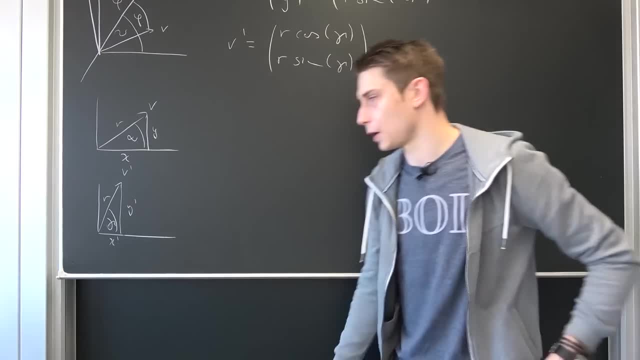 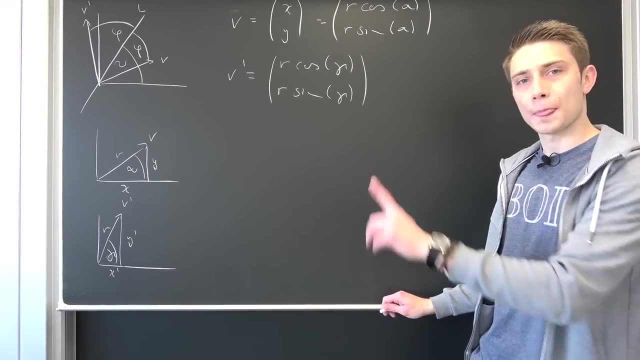 with the angles. that's the only difficult part. you could say. I for myself like to mix up stuff and then I'm not arriving at what I actually want. So I'm going to take a look at the x-axis. Let's say we want to arrive it, but we are still going to give it a shot. 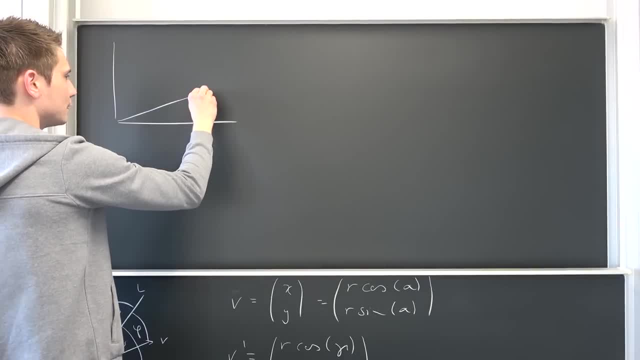 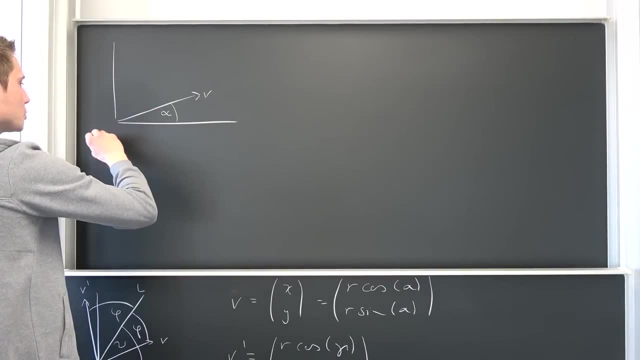 Once again we have a coordinate system right here. we have a vector v right here with an angle alpha, enclosed here between x-axis and our vector. Also, we have this line l being spanned out right here and between our v and this line l we have 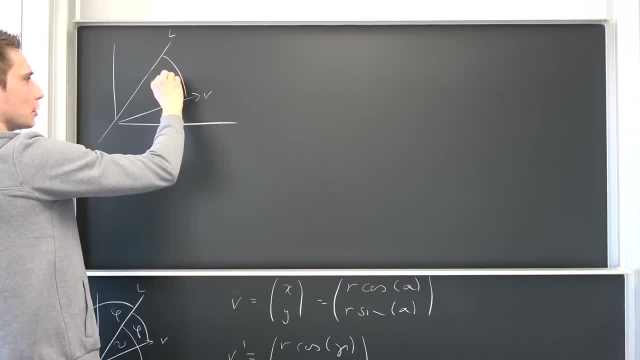 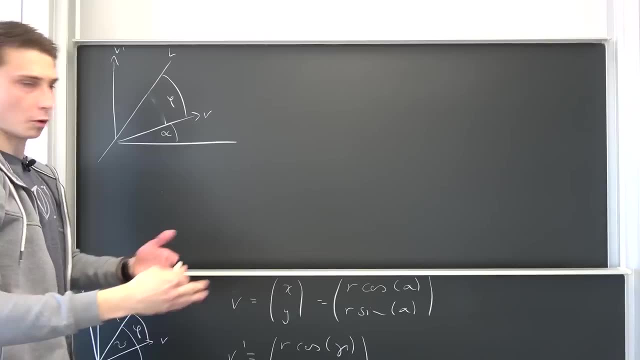 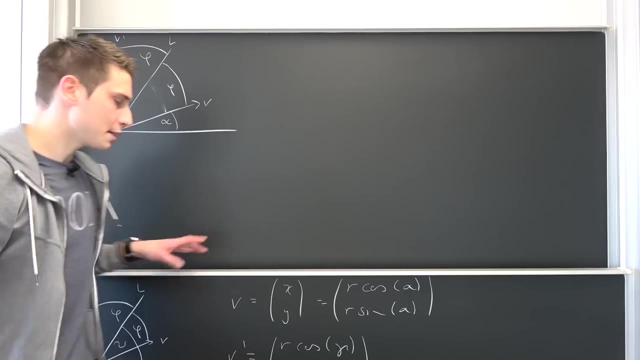 a certain um, we have a certain angle. let's call it phi, just like before. Also, let's say we have v prime, that's the reflected vector right on the y-axis, for example, also enclosing this angle, phi, Like I said, our reflection matrix is going to tell us. 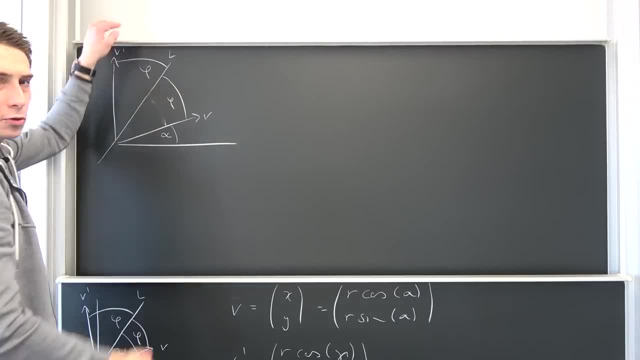 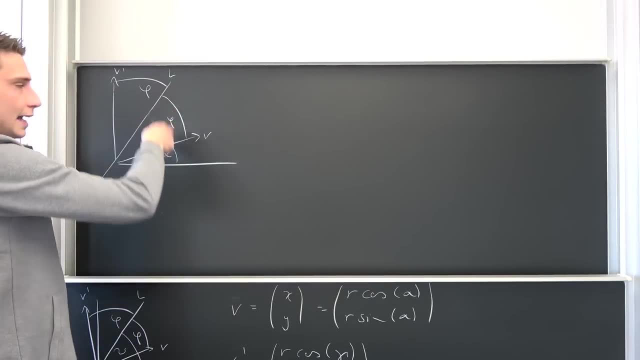 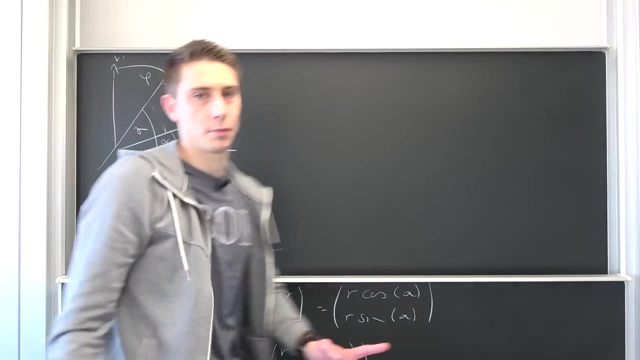 exactly where our reflected vector v prime is going to be after we've applied this line right here, having a certain angle between our l line and our x-axis- Let's call this thing right here- I really don't care- fader, for example. Okay, now we can do some trigonometry right here, some. 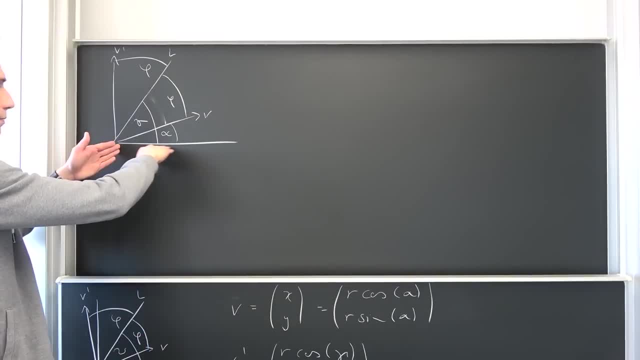 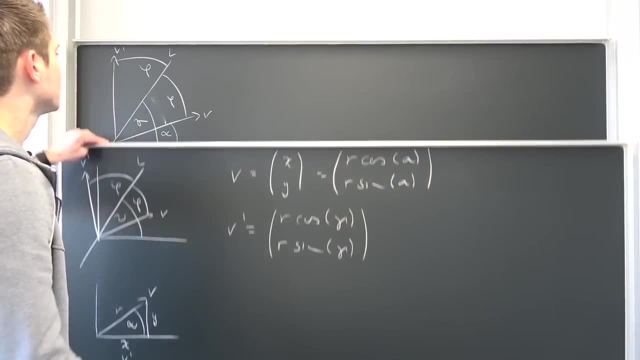 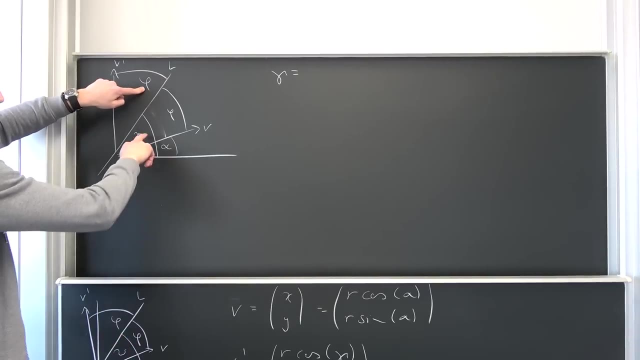 angle playing around, because you know, this angle right here between our x-axis and our vector v prime is exactly our gamma that we have proposed right here. Okay, so our gamma. what is it going to consist of? Well, it's going to be just phi plus fader, right here. 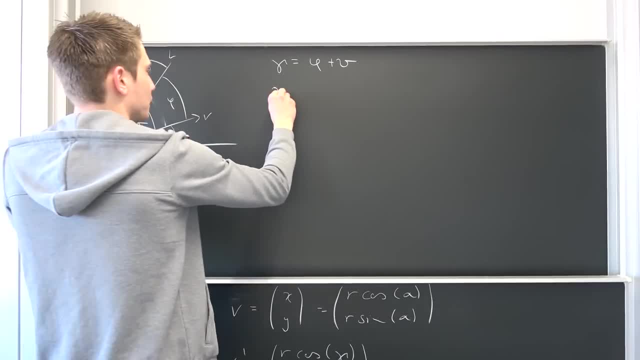 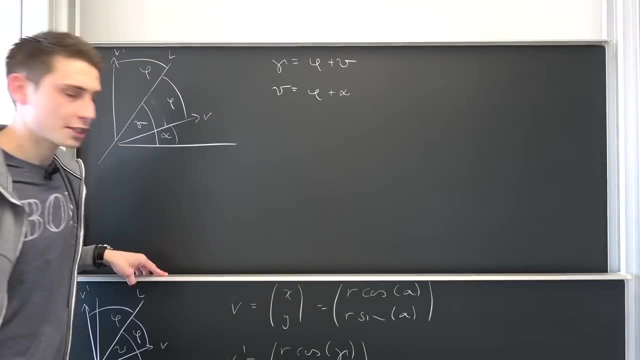 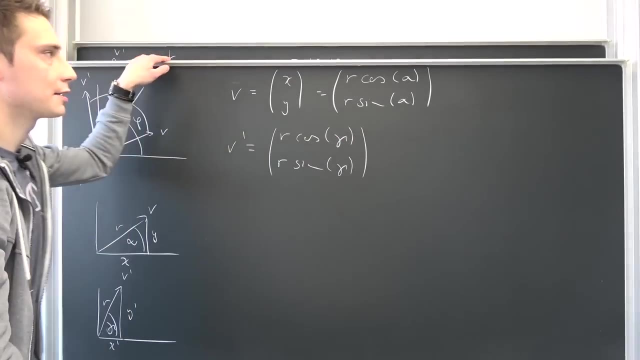 Also what, for example, is our angle fader? Fader is nothing but well, phi plus alpha, and, just like we did with the reflection matrix, we want to kind of substitute our original vector in in the end. So our angle gamma that we have to find out has to consist of our reflected 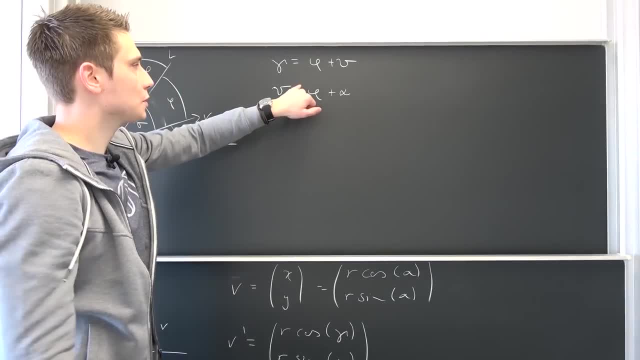 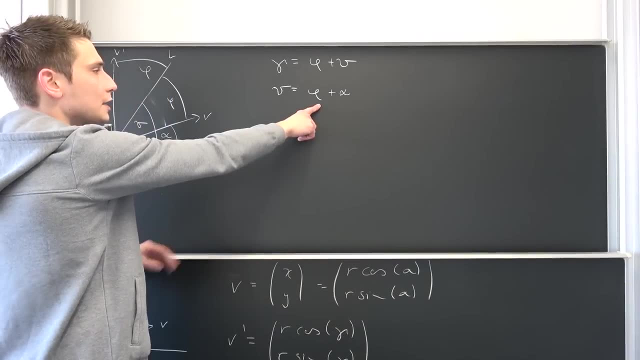 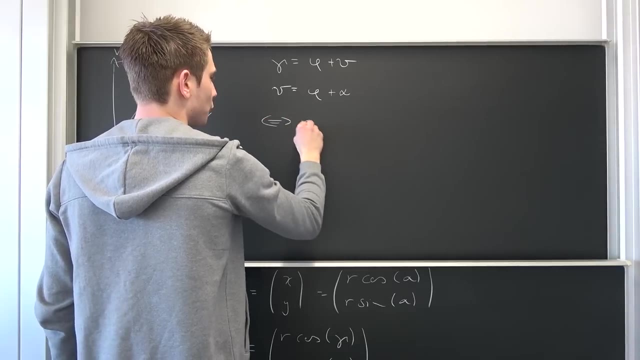 angle, you could say, of our line l and also um with regards to our alpha, because we want to substitute this right here in. So why not solve this thing right here for phi, so that we can substitute phi into here, meaning phi is nothing but fader minus alpha. We can substitute this value. 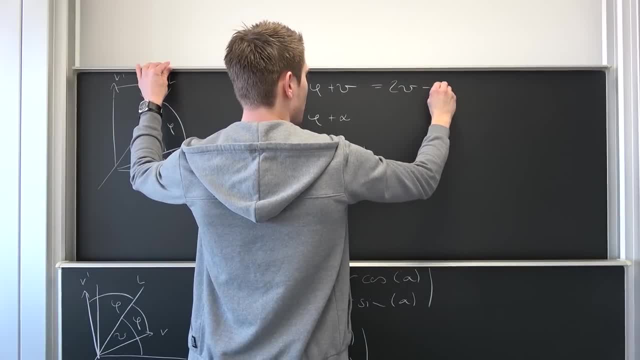 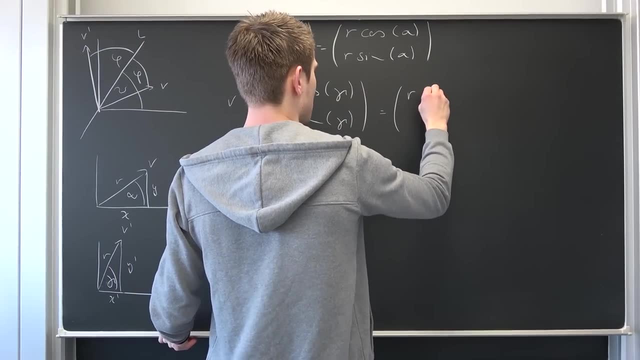 into here and get that um. 2 times fader minus alpha is nothing but gamma. Okay, that was actually quite easy. we can plug this into here. That's nothing but r times the cosine of. okay, 2 times fader, the reflection angle minus alpha. 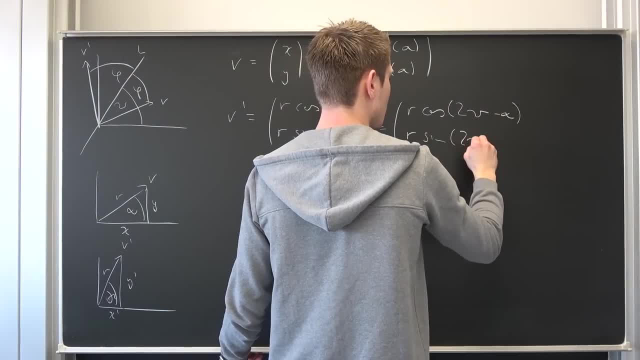 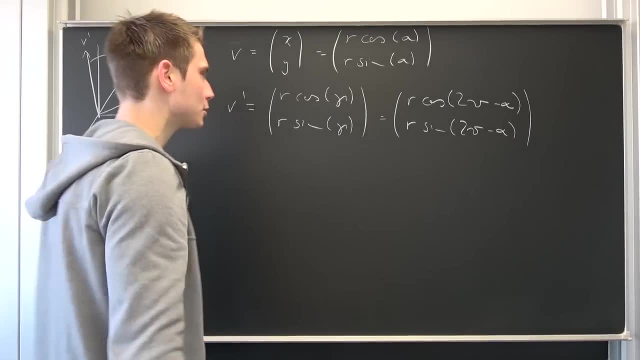 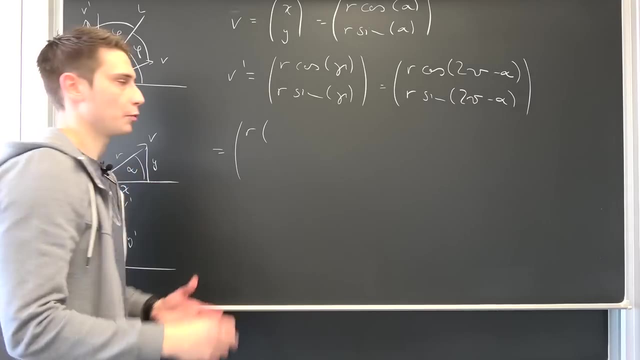 And r times the sin of two times fader minus alpha. And, just like with our rotation matrix, we can actually use addition formulas right here. We're going to end up with a big s vector right here. r Okay, now we can just use the addition formula for the cosine, just with a sin switched in the end. 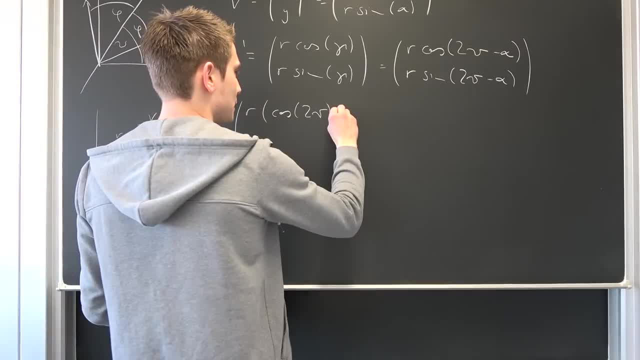 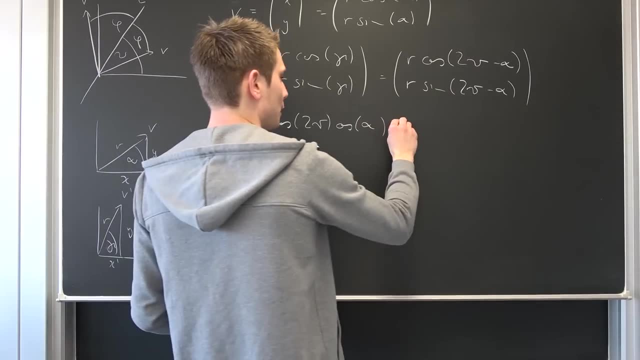 So this is the cosine of 2 times fader. just write a list of addition formulas: times the cosine of negative alpha, of negative alpha. but this is just cosine of alpha. you could say Okay and then in the normal case you would have negative. I'm going to write it out then. 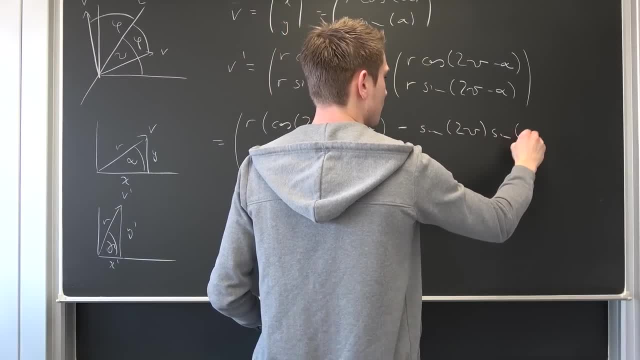 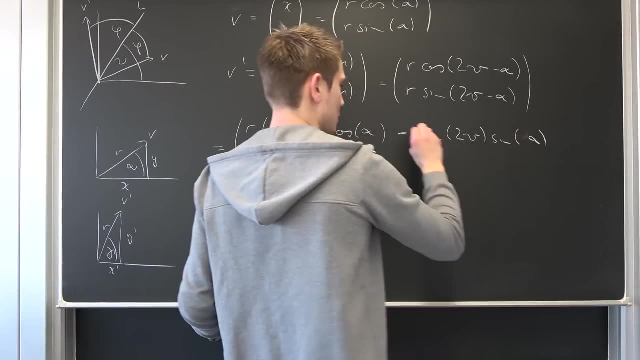 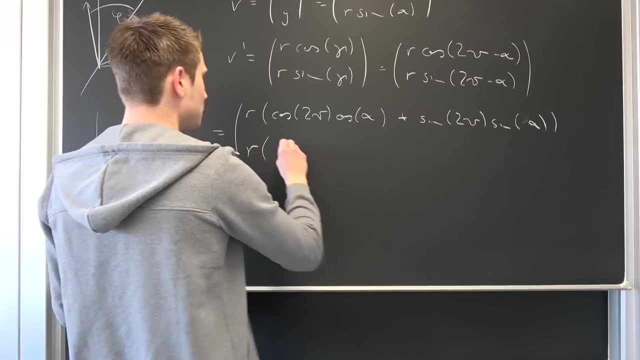 we have the sine of two times theta, sine of negative alpha, but the sine of negative alpha is nothing but this negative sine of alpha, so we can bring this to the outside. that's where we get this positive sine from. Okay, now we have our times. Okay, cosine of two times theta, times the sine of negative alpha, and 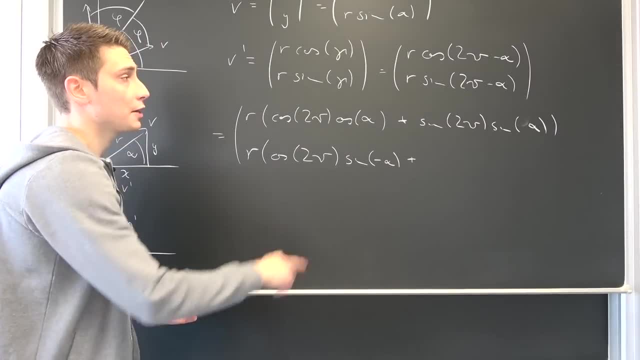 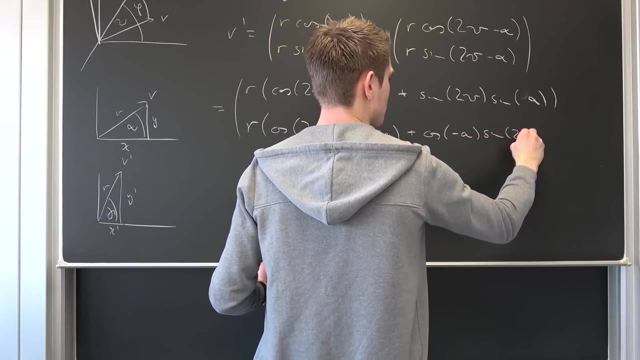 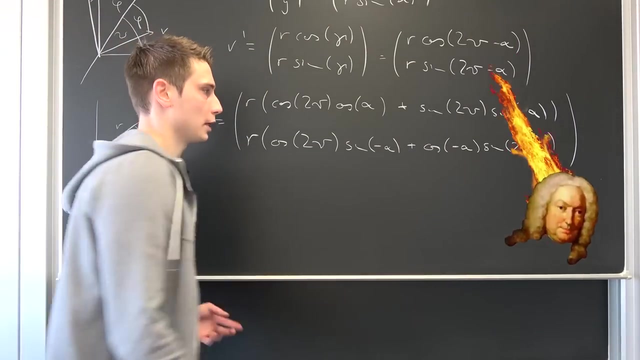 then we have positive sine right here in the addition formula, in the normal case, and then we have the cosine of negative alpha times the sine of two times theta. Closing of everything. Cosine of negative alpha, well, it really doesn't quite matter, it's just cosine of alpha, it's an even function. but we 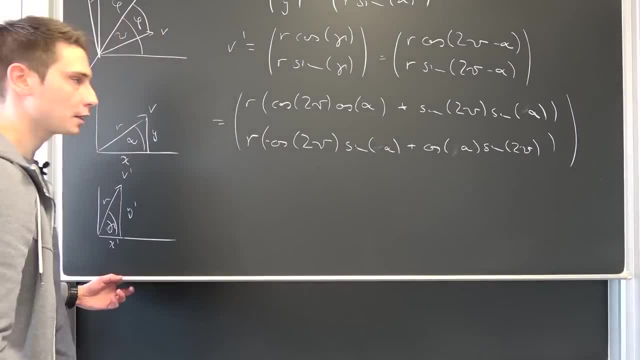 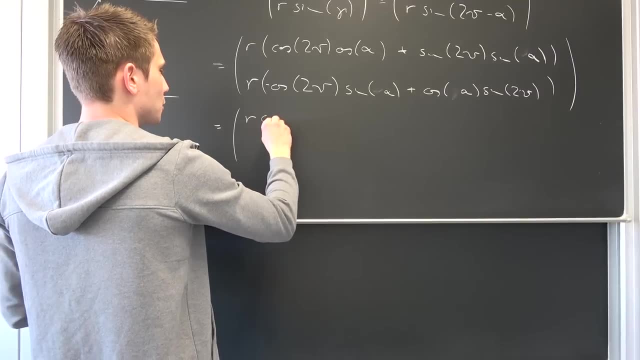 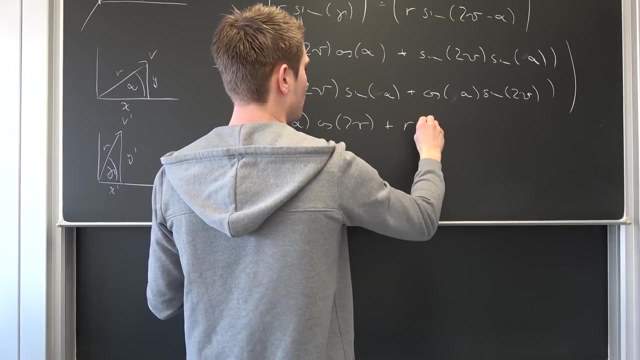 can drag this negative sign, just like before, to the outside. We're going to get- let me just sort everything a little bit At first we're going to get- R times, the cosine of alpha times, the cosine of two times theta plus R times the sine of. 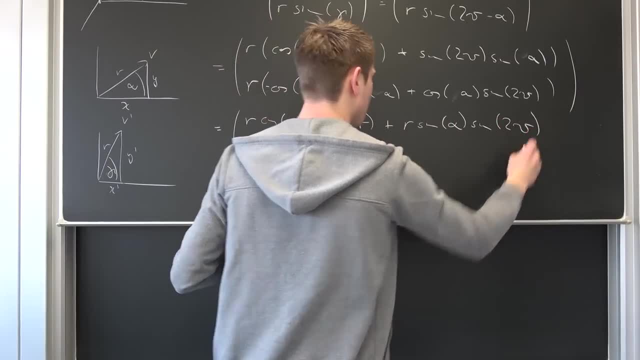 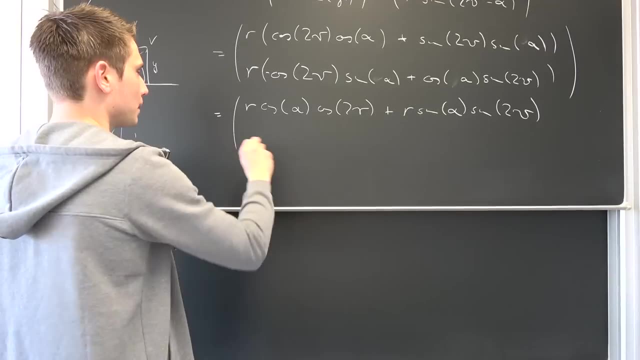 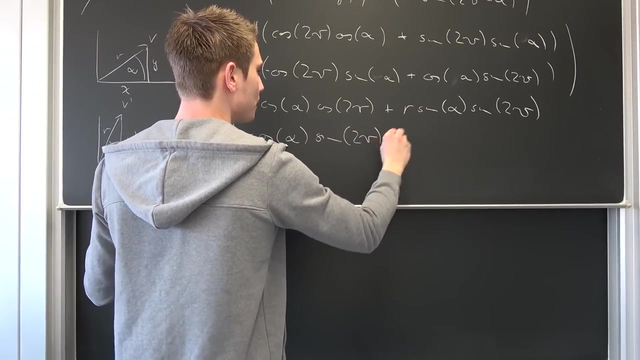 alpha times the sine of two times theta. Down here we are going to get: okay, let me bring this in a different order. I'm going to distribute it into here and then we are going to see what you get. This is nothing but R times the cosine of alpha times, the sine of two times gamma. negative sine R. 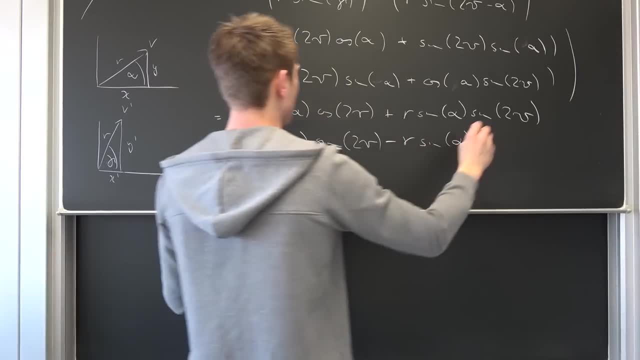 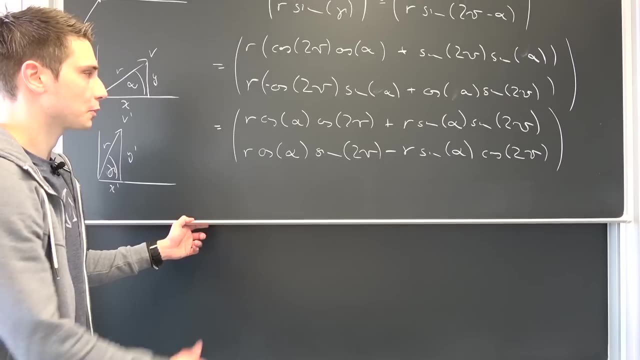 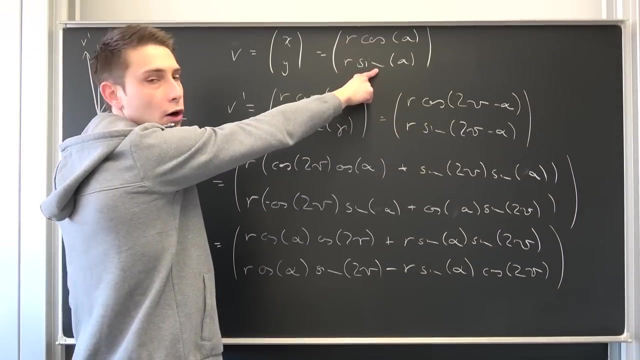 times the sine of alpha, times the cosine of two times theta. Okay, here we go. that's actually quite good, because R times the cosine of alpha is nothing but our original x-coordinate, and R times the sine of alpha is nothing but our original y-coordinate, Meaning we're going to 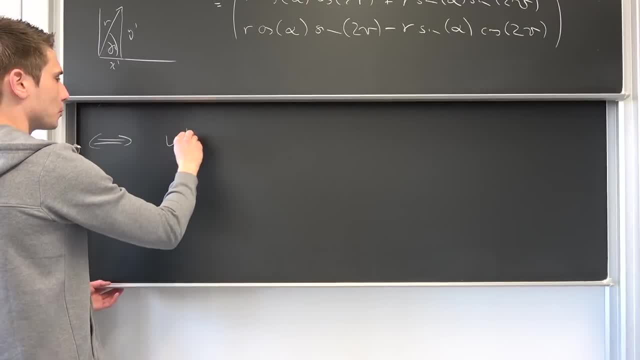 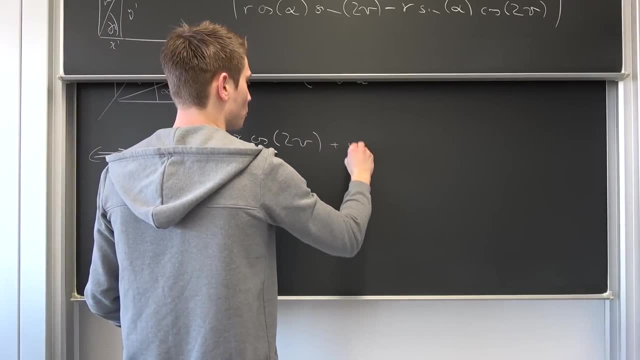 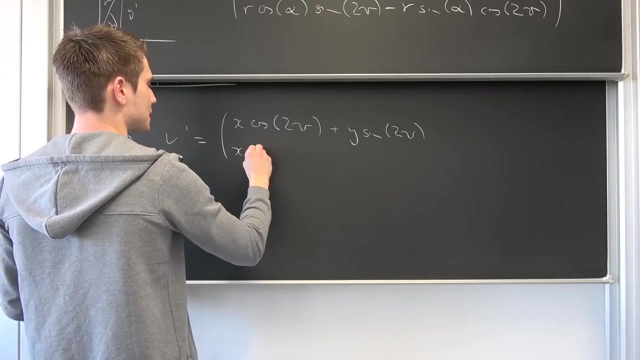 get overall that v' is now nothing but okay. this is: x times the cosine of 2 times theta, plus y times the sine of 2 times theta. x times the sine of 2 times theta, minus y times the cosine of 2 times theta. 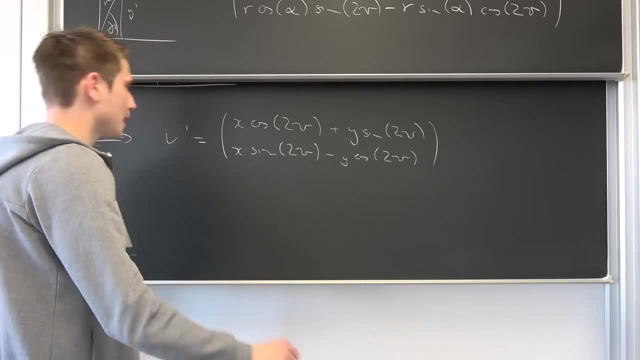 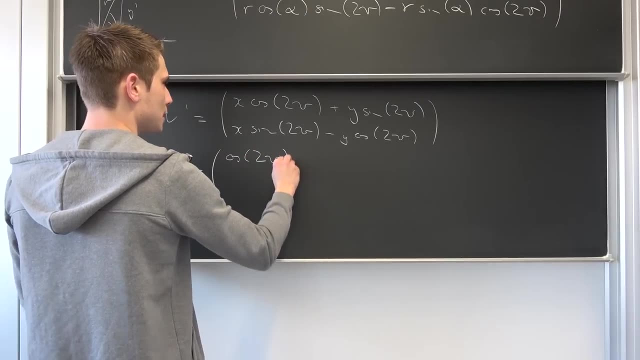 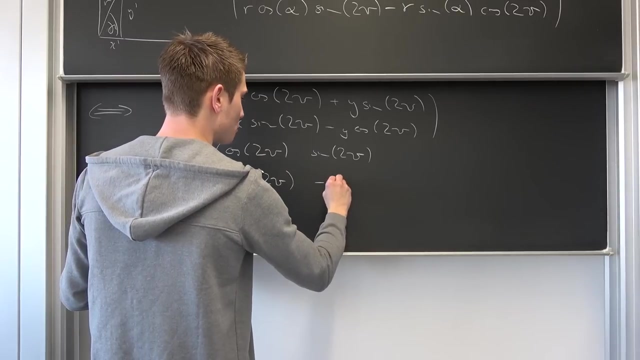 And now we are going to let some vector calculus magic happen, namely this thing right here is nothing but some matrix, namely cosine of 2 times theta sine, of 2 times theta sine, of 2 times theta minus, cosine of 2 times theta multiplied by x and y vector. 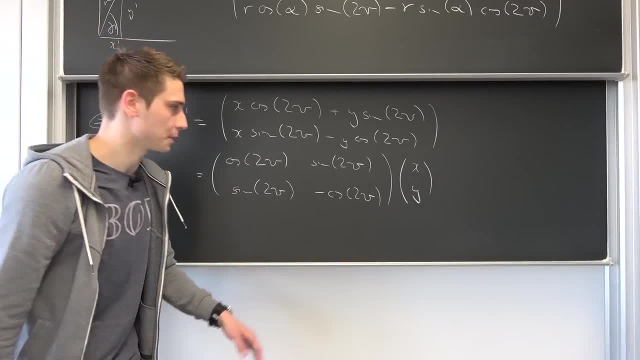 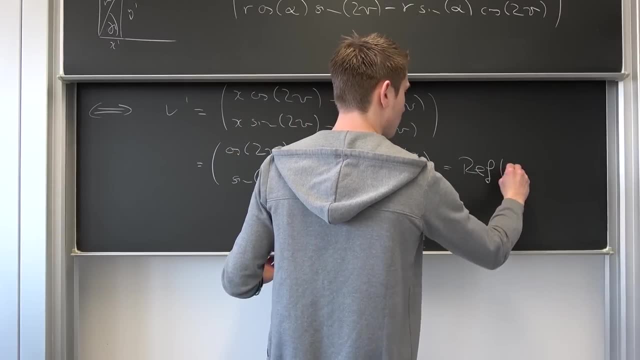 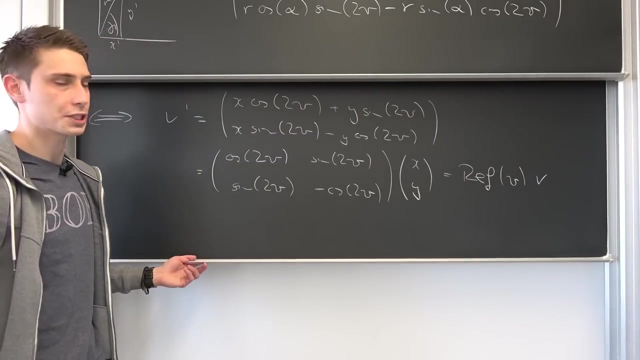 Cool and that's really quite good, because, you see, this right here is actually our reflection matrix that we wanted to get. So this is nothing but the reflection matrix, Where we reflect, Reflect by an angle of theta times, our well v, in this case, our original vector. 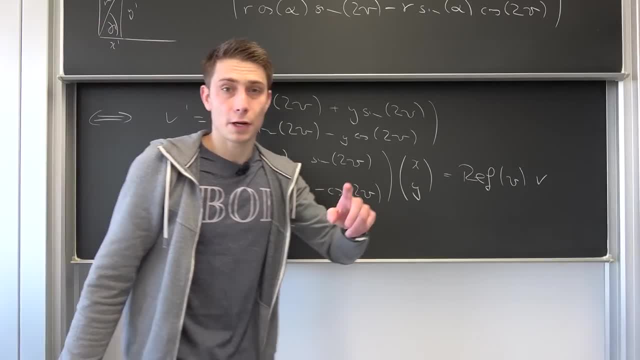 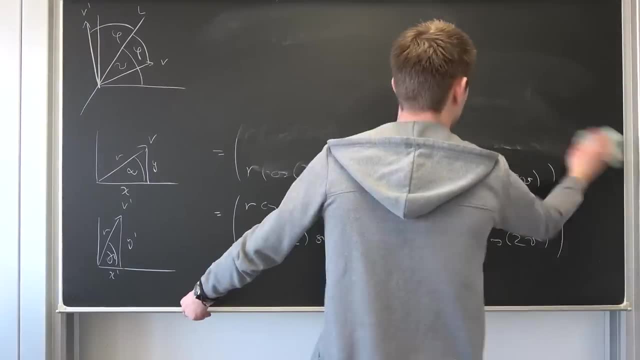 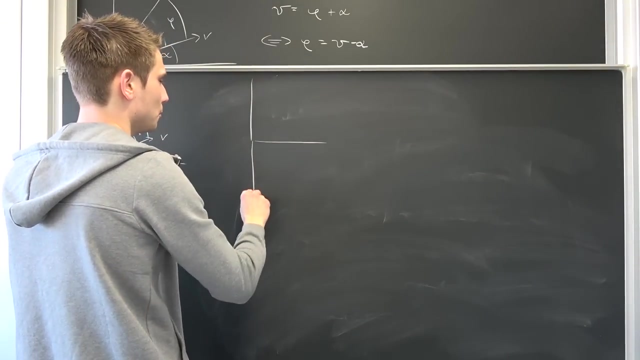 There are many applications of this right here, For example. why not take a look at the complex plane, for example? Let me erase a little bit. So what's an application? Let's say we have a vector right here in the complex plane, okay, and this vector is for: 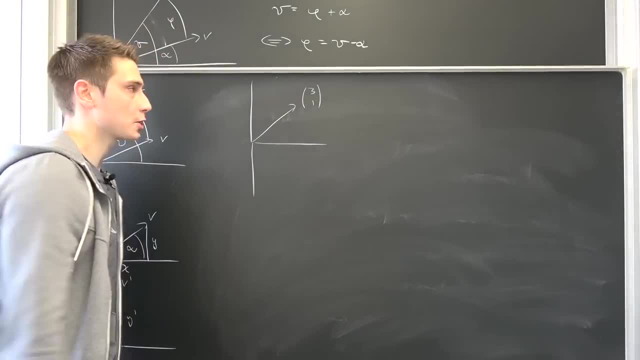 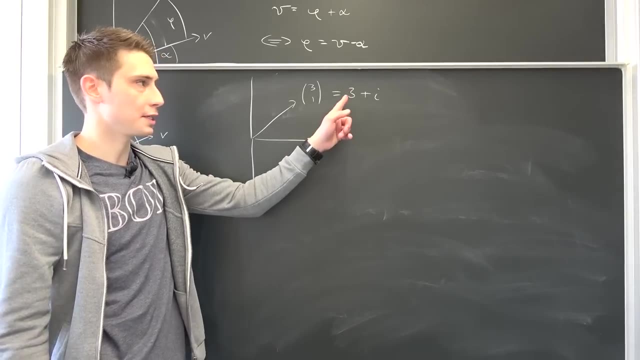 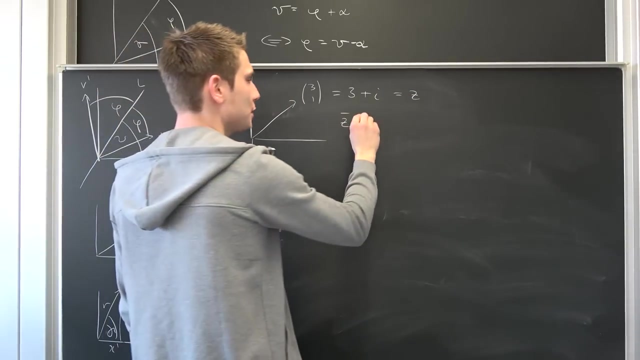 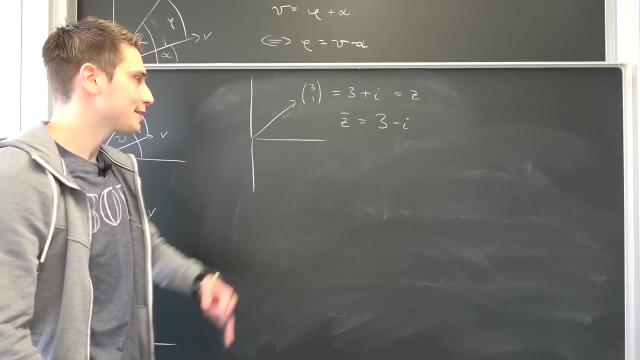 example 3 and 1.. Okay, that's a complex number, corresponding to 3 plus i, for example. Now what we want to do? we want to find its complex conjugate. meaning z, line, z, hat. whatever. the complex conjugate is nothing but 3 minus i, meaning, geometrically seen, that we are. 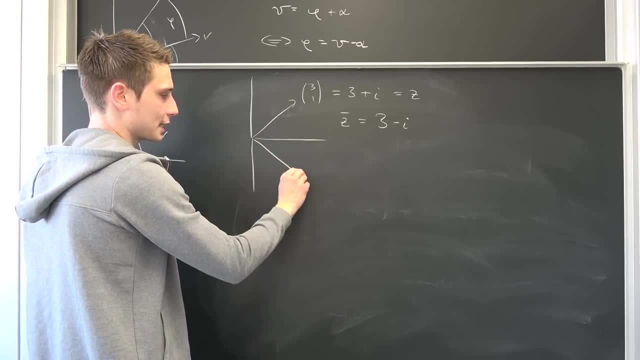 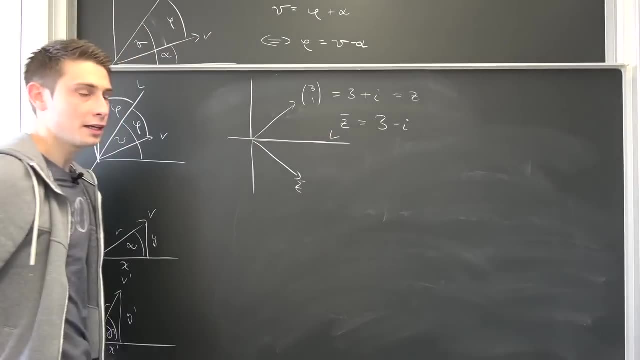 going to reflect it that thing right here on the x axis. That's our complex conjugate down here. Meaning, if we would interpret our x axis as our line L, this line L and the x axis are going to enclose 0 degrees Celsius. 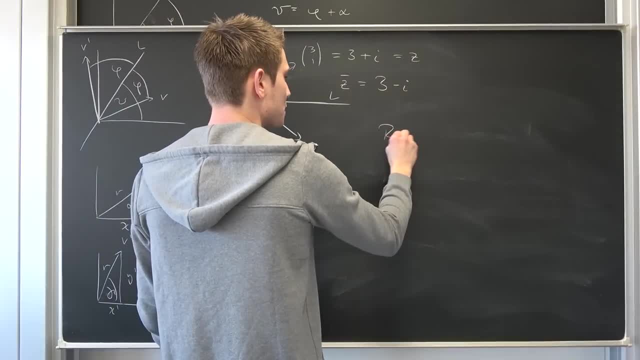 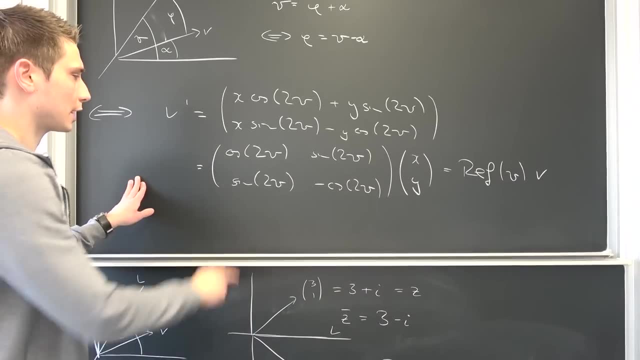 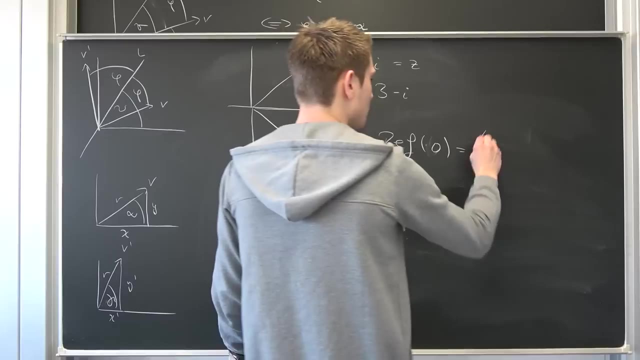 So 0 degrees overall, meaning our reflection matrix of 0 in this case. okay, we are going to use this is going to be okay. cosine of 0 is just 1.. That's going to be 0 and this is going to be negative 1.. 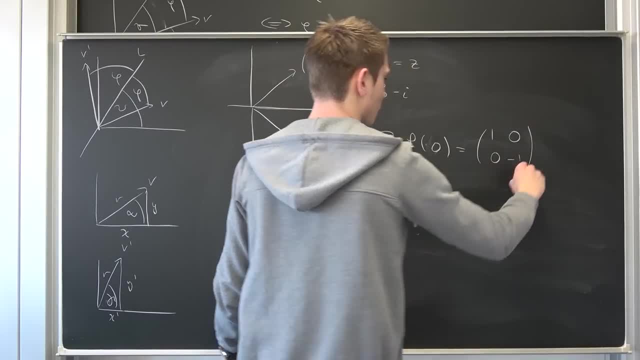 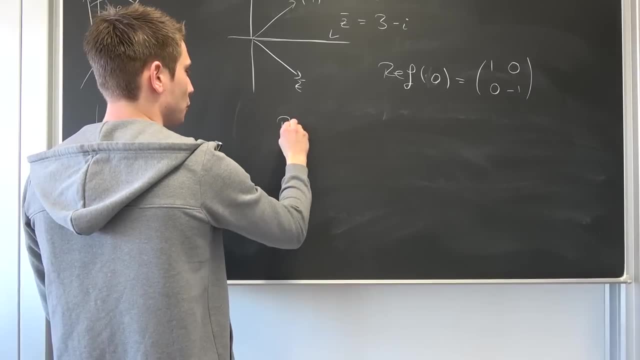 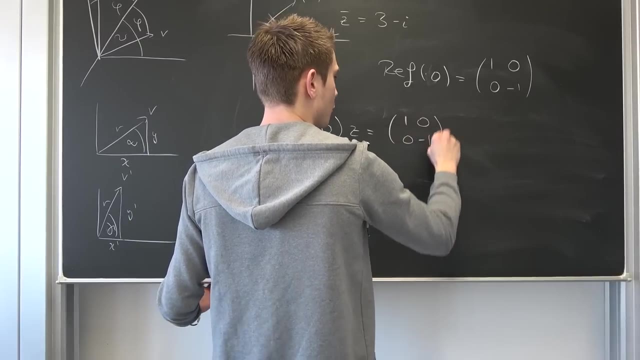 Meaning. we have a matrix, 1.. 0.. 0. Negative, 1.. If we apply this vector right here, this complex number, to this reflection matrix, so reflection of 0 times our z, we are going to get okay: 1, 0, 0, negative, 1, 3, 1, okay. 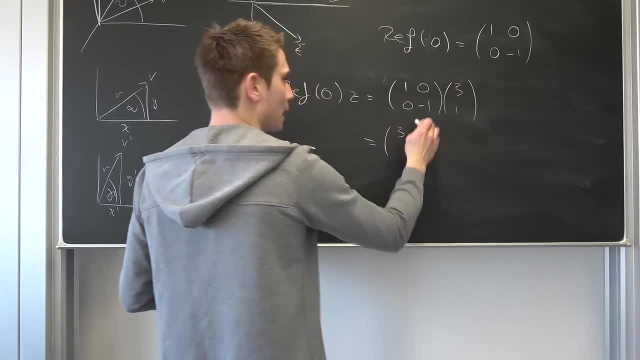 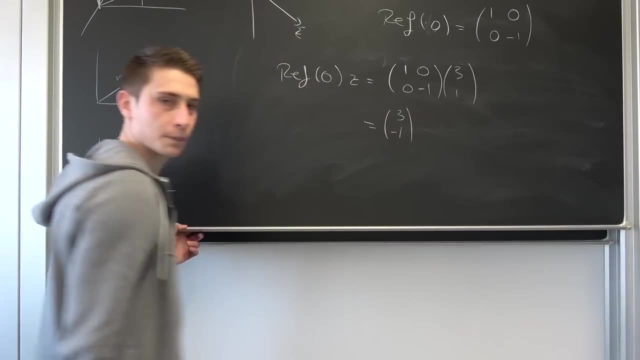 If we apply this, we are going to multiply this together. we are going to get 3 up here. so 3 times 1 plus 1 times 0 is going to be 3.. This together, we are going to get negative 1.. 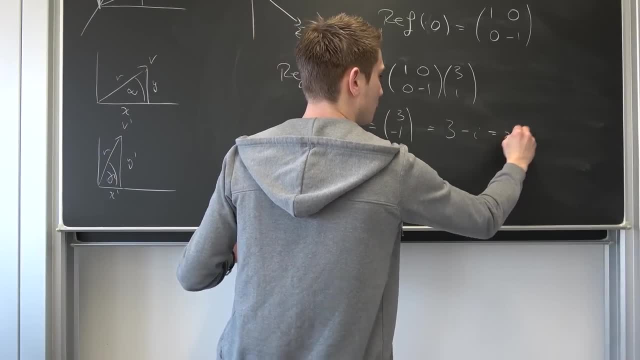 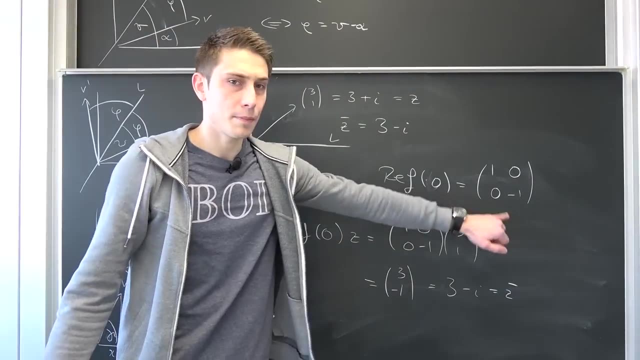 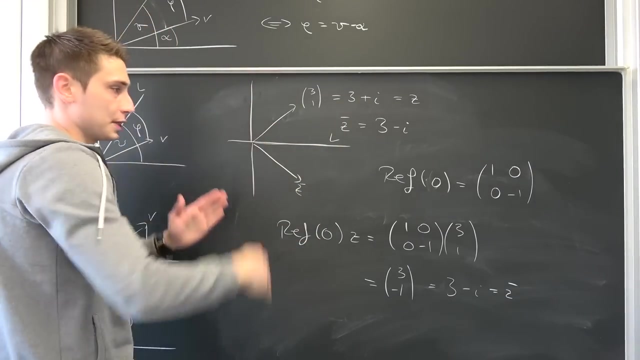 And this is exactly our complex conjugate. So you see that that's actually quite a good application of this thing. You can find those standard matrices for those standard reflections, for example the line L lying on those on this y axis, or for example here: 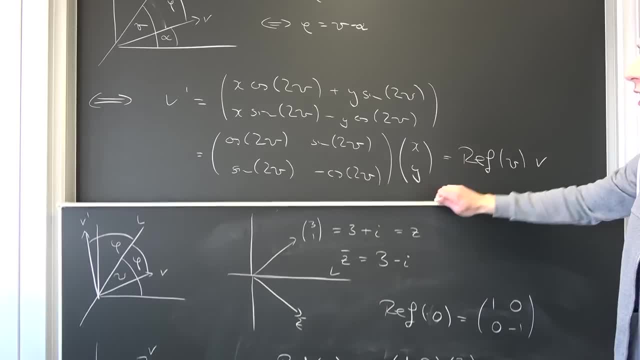 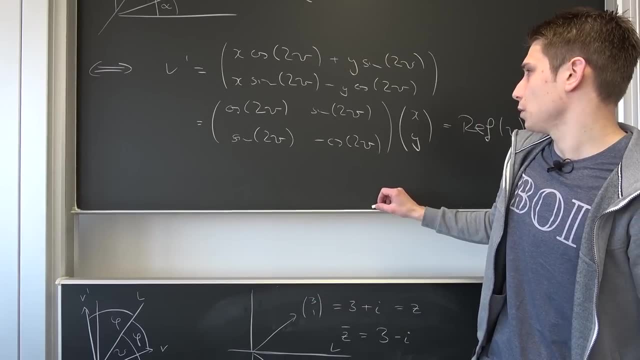 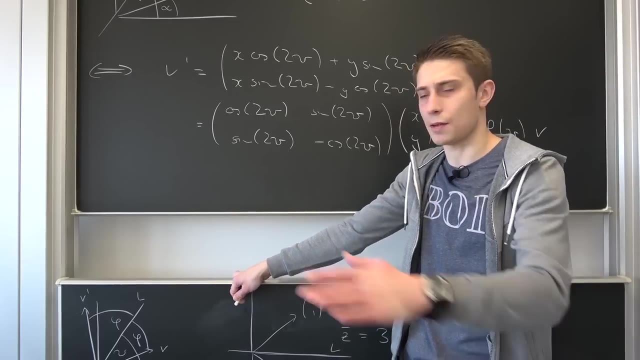 But yeah, this is basically it, This is our reflection matrix, and it's quite useful. actually. I've seen it popping up in experimental films, I've seen it popping up in experimental physics, But I'm not sure anymore. I guess it had something to do with polarization Jones matrices or something. 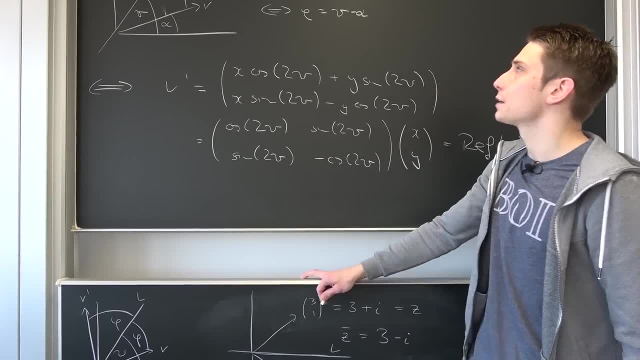 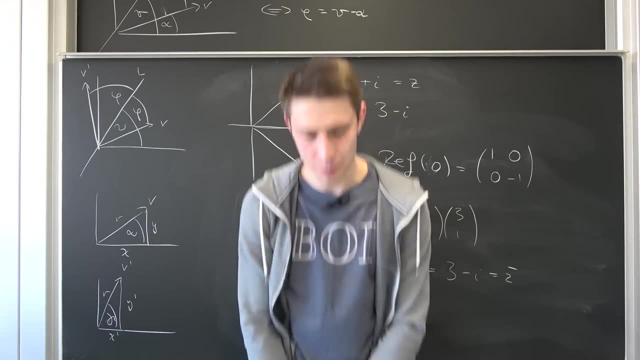 I really don't remember. But yeah, it came up somewhere and I just derived it yesterday because it sounded interesting. And yeah, there we go. I thank you guys for watching. If you did enjoy this video, please like and subscribe and recommend the channel. 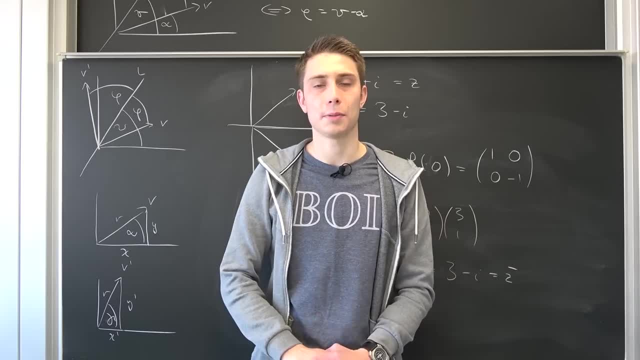 If you want to support the channel a little bit more, you know how you can do this And, up until the next video, have a flammable day. See ya Peace. 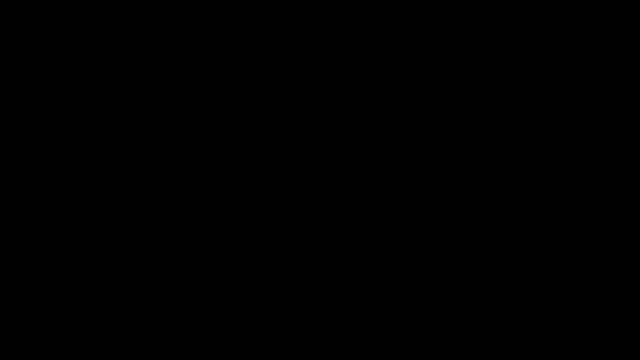 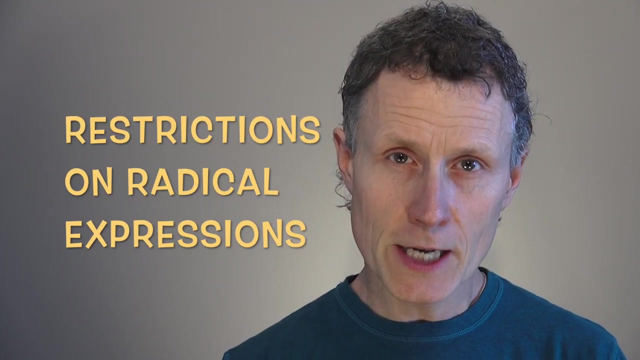 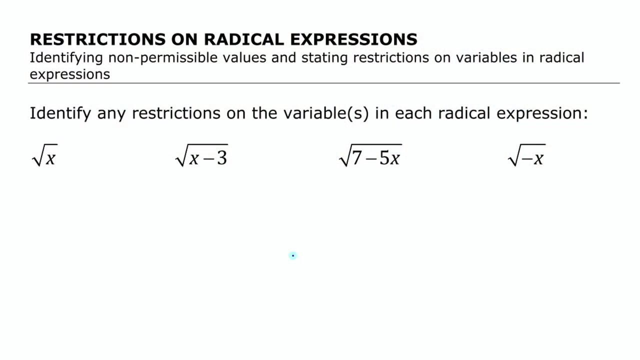 Hey there, In this video we are going to look at restrictions on variables in radical expressions. In other words, we're going to look at if there are any values that are non-permissible for those variables. So if we're going to look at radical expressions with variables, 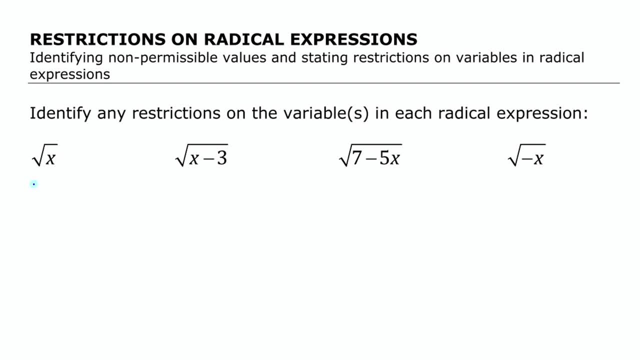 in them, like any of the ones there. we need to think about the values of the variable that allow the expression to be defined, Or in other words, are there any non-permissible values? Are there any restrictions we need to think about on the values of the variable?